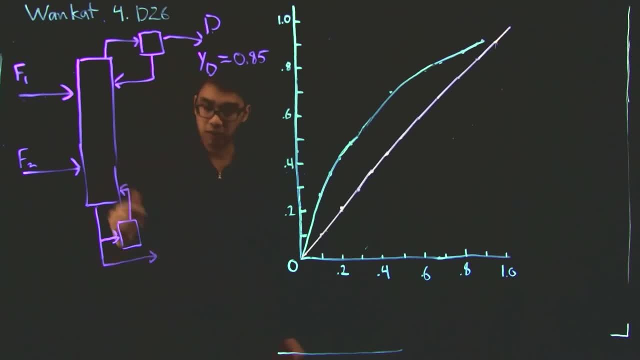 The remainder is the bottoms, and this has a composition of 10% acetone. Let's talk about the feeds. The first feed we have is superheated vapor at a flow rate of 100 moles per minute And the composition is 50% acetone. 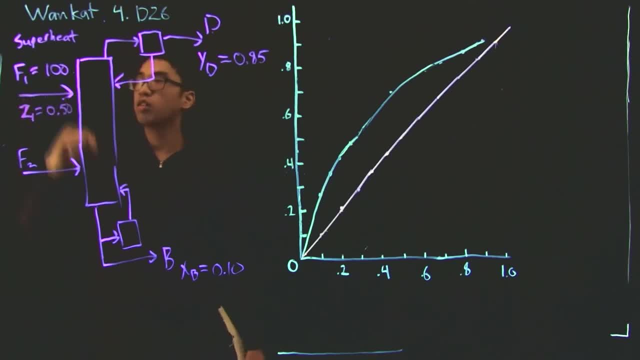 We know that for every 20 moles of vapor, we require one mole of liquid to evaporate in order to lower the temperature to desaturation temperature. Next, we have a second feed, which is a saturated liquid at 150 moles per minute. 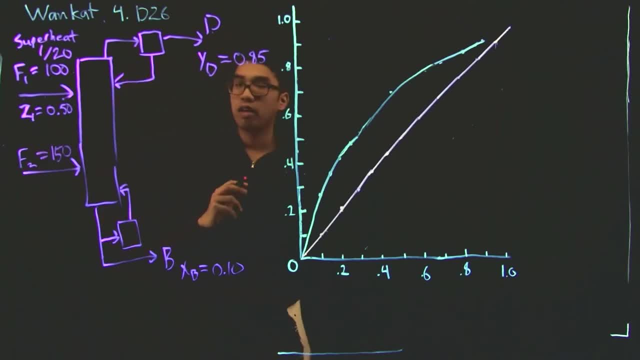 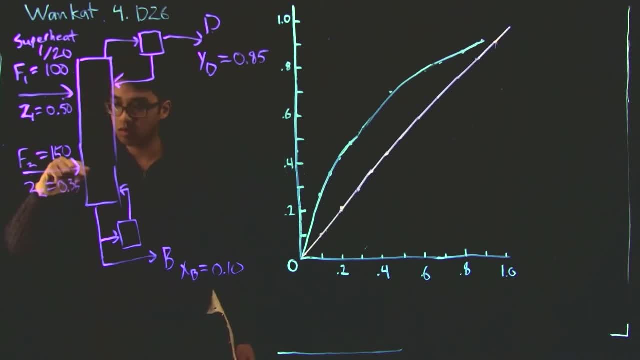 which is 35% acetone. Now what we're tasked with finding is the V bar over B ratio. is the V bar over B ratio the minimum ratio, ratio, minimum ratio. Now, to do that, we need to find all of the internal load. 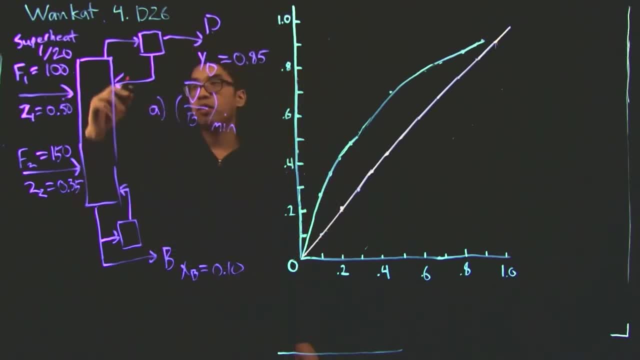 internal flow rates. So let's start by just labeling everything. So here we have V, Here we have L, And then for the bottom we're going to use V bar and L bar, And obviously we have V And because we have two feeds in. 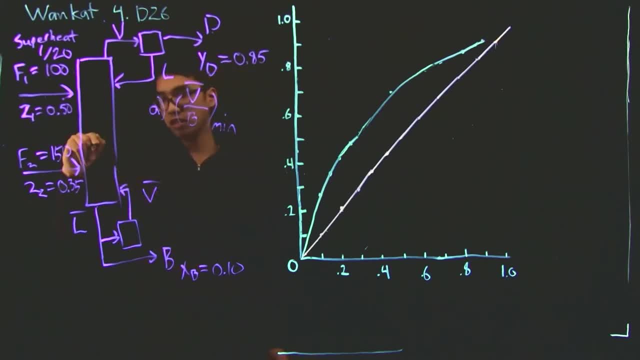 between the two feeds, there's going to be a first set of internal streams, which we'll label V prime and L prime. Now the next step is to perform a total mass balance, And so we know that F1 plus F2 is equal to D plus B, And 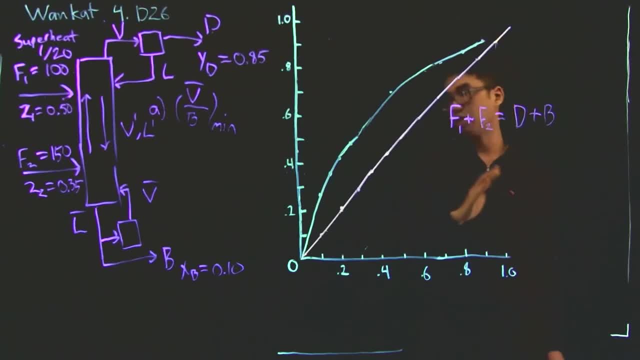 since we know F1, F2, we have two unknowns, so we need a second equation to solve it, And we can do that with a component mass balance. So we have Z1. F1 plus Z2. F2 is equal to y, D, D plus x, B, B. 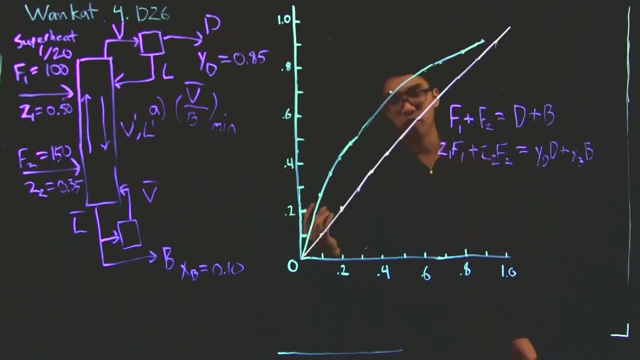 Now, when you actually substitute in the numbers, you get 2.. 250 is equal to D plus B, And over here you get 0.35 times 150. plus 0.50 times 100 is equal to 0.85.. 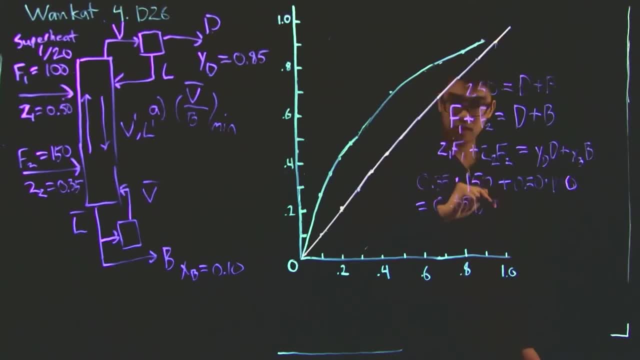 D plus 0.10B, And so when you solve this, you will obtain the values V. Sorry, D is equal to 103.3 volts per minute And d is equal to 146.6 mols per minute. Unfortunately now we can't make any further progress. 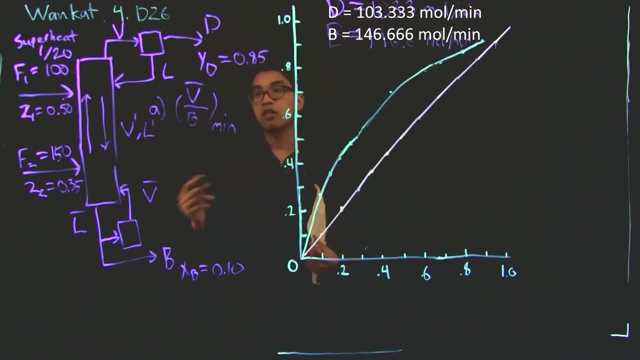 because obviously we don't have v-bar over b-min and the flow rates at the top are driven by equilibrium, so we don't really have a way to calculate them. So the next step here is to calculate the feed lines And, as a reminder, the feed lines are given by the equation: 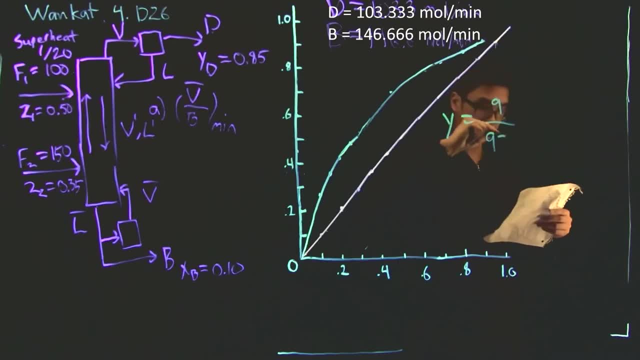 y is equal to q over q minus 1, x plus zf, 1 minus q. The first step in calculating the feed line is to determine the value of q. Now, q is the feed quality and it is the fraction of the stream. 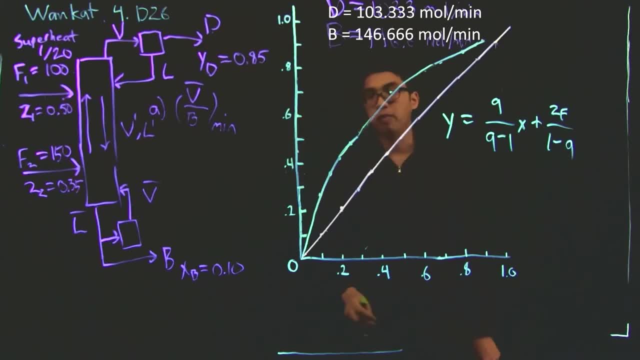 that remains liquid after it's been fed into the column. So for F2,, F2 is a saturated liquid, so the whole stream is liquid, and so q2 is equal to 1.. Now q1 is a bit more complicated. 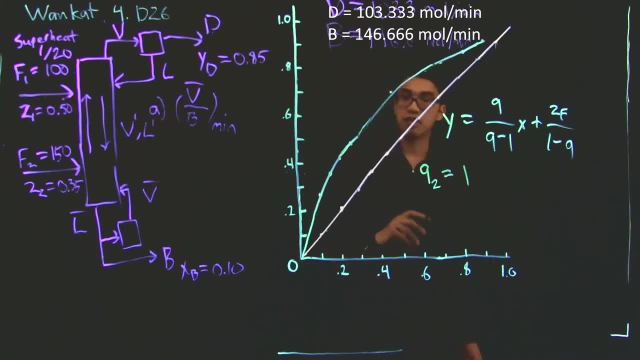 Because it is a superheated vapor, and so not only is none of it going to be liquid when it's introduced into the tower, it's also going to convert some of the liquid into vapor, And so, because of that, this q is actually a negative value. 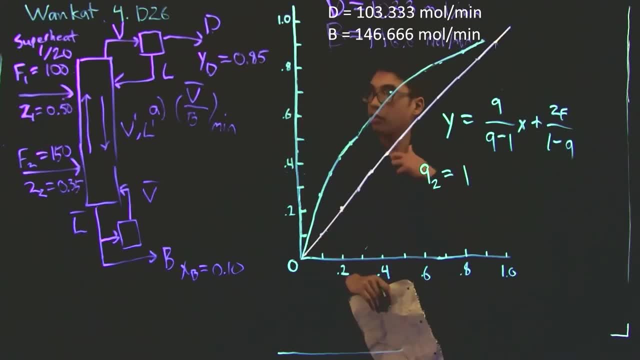 And the negative value is going to be dependent on how much liquid is evaporated. So in this case, for every 20 moles of feed, one mole of liquid is evaporated, And so the value of q is going to be: q1 is equal to minus 1 over 20,. 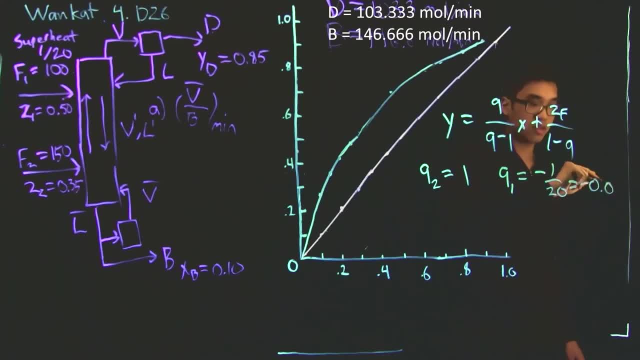 which is equal to minus 0.05.. Now let's calculate the feed lines For q2, for the second feed, since it's a saturated vapor, this term is going to be: this denominator is going to be 0. And so the feed line is going to be a vertical line. 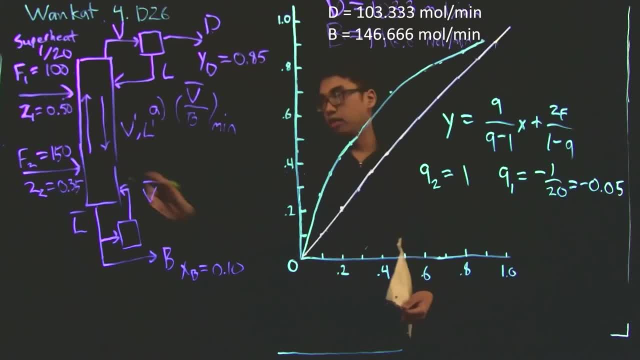 that passes through the point z equals 0.35.. So that would be about here, And so we can say that we can show, and so the feed line is just going to be a vertical line like this. Now for the second, for the first feed. 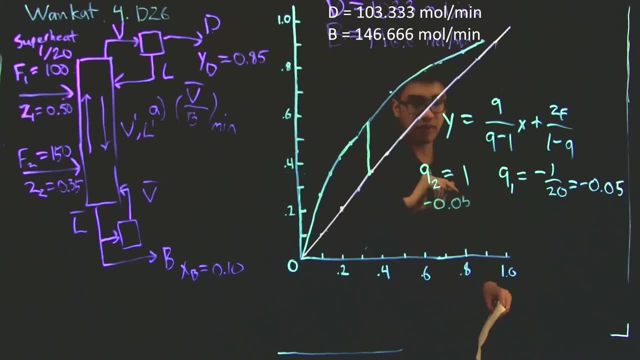 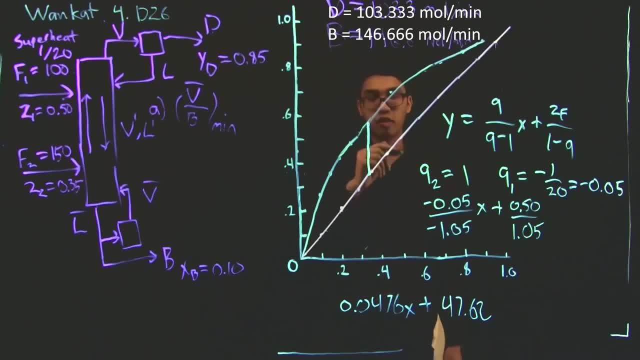 So this slope here is absolutely tiny, so it's very, very close to a horizontal line. We know that it will pass through the point z equals 0.50, so we can go ahead and draw that, All right. So we know that the y-intercept is 47.62,. 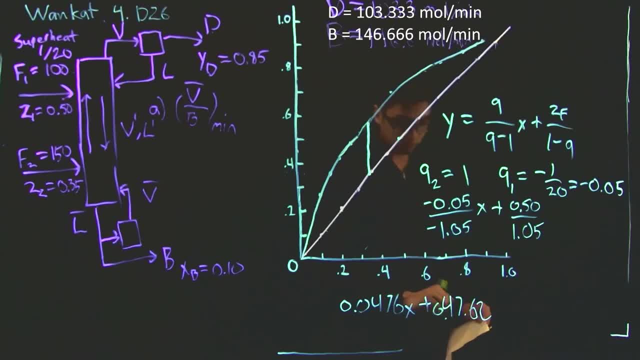 well, 0.4762.. And so it's going to be roughly here, And so we just draw a quick, a quick line. It's going to look like this: The next step is to estimate v-bar over the y-intercept. 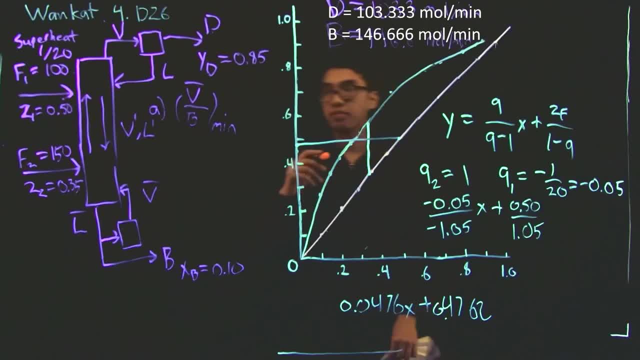 So we're going to estimate v-bar over b-min by examining the graph. Now we know that at v-bar over b-min, or the minimum reflex ratio, the operating lines will form a pinch point. So upon examination there's two points where they can pinch. 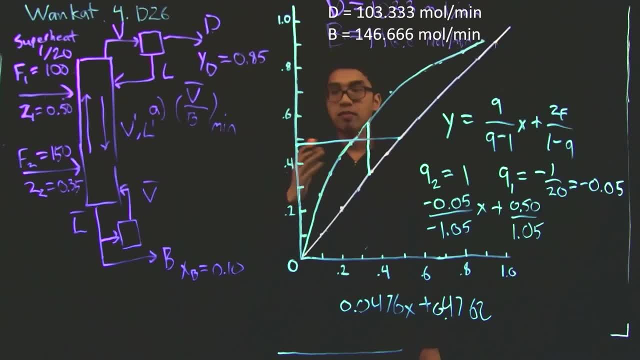 here or here Now, at v-bar over b-min, we know that the lower operating line is going to have its deepest possible slope. So because of that, we know that the pinch point we're going to choose is this one. So we're going to draw an operating line. 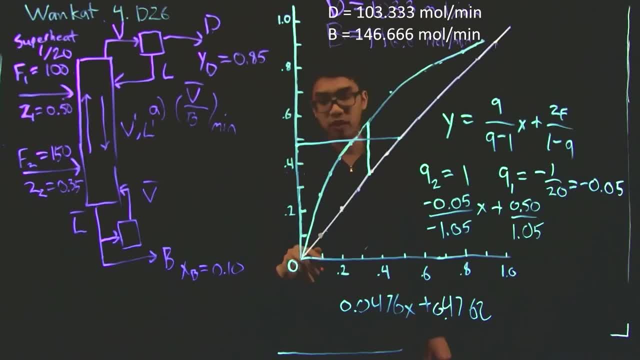 that starts at xb equals 0.10.. And it's going to run from there to the pinch point. So this is not the best line, but you get the idea. And so after that we know that the operating line equation is: l-bar over v-bar x plus l-bar over v-bar minus 1xb. 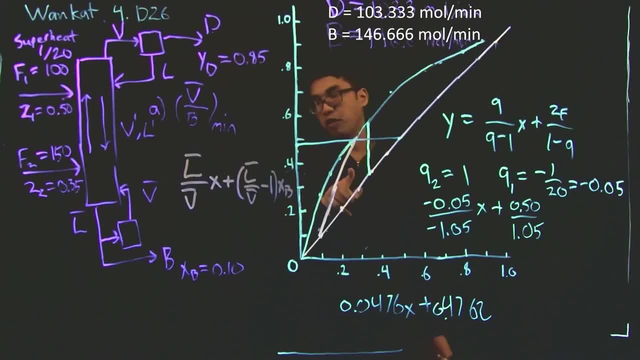 And so by measuring the slope of this operating line, we can find l-bar and v-bar, And then after that it's a fairly trivial calculation to find v-bar over b. So let's look at this, Let's do that. So if you take this operating line and you measure it, 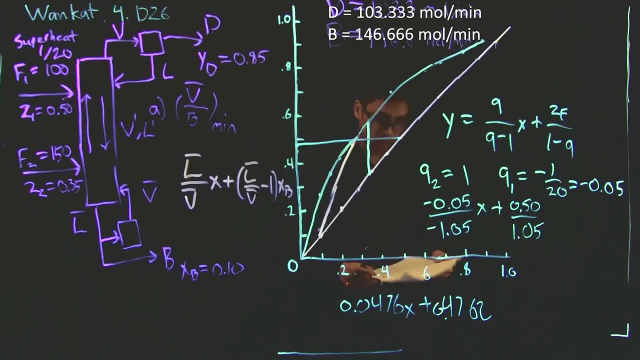 you'll find that the slope is approximately equal to 3.. So l-bar over v-bar is approximately 3.0.. Now the next step obviously is to just calculate v. So we know that from that if we rewrite it. 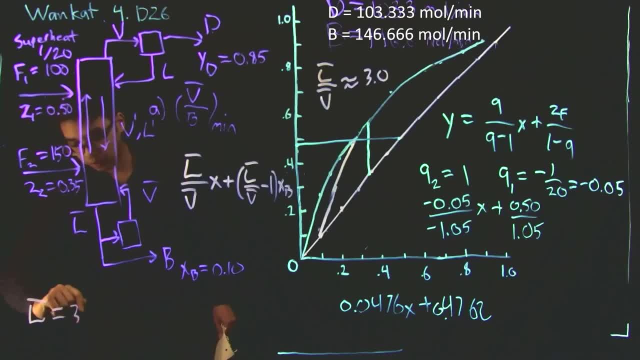 we know that l is equal to 3.0 times v-bar. We also know that l is equal to v-bar plus b. So if we substitute this in, we'll find that b is equal to 2, 2 times v-bar. 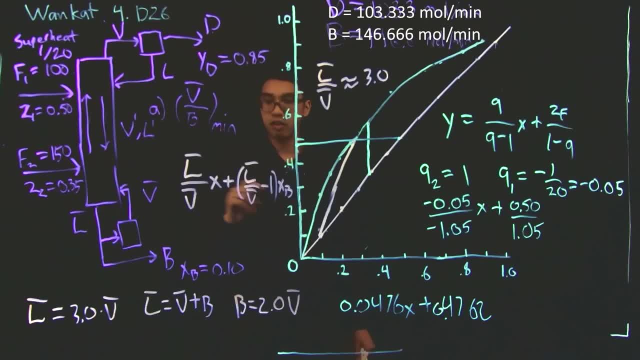 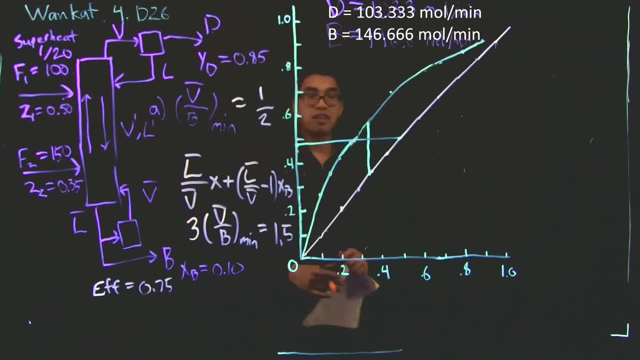 And so, therefore, v-bar over b is equal to 1 half. Okay, so we know that 3 times v-bar over b-min is equal to 1.5.. And now we need to find the other flow rates. We know that b stays the same because it's still 146.6 volts per minute. 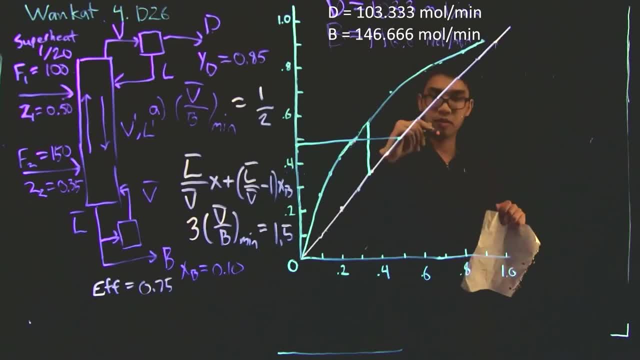 And so we'll have to back-calculate. So we know v-bar over b is equal to 1.5.. And therefore v-bar is equal to 1.5b, which is equal to 1.5 times 146.66,. 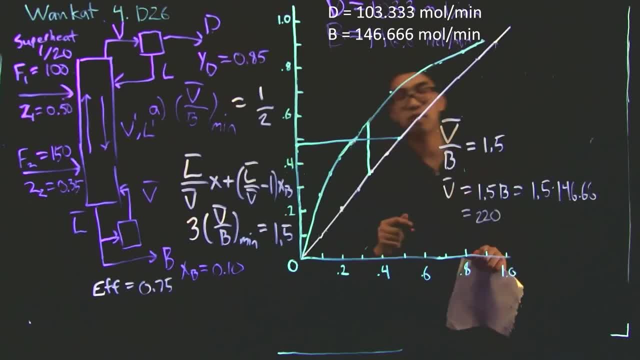 which is equal to 220.. Next, l-bar is equal to v plus b, which is equal to 1.25b, And this is equal to 366.66.. Taking all that, we find that l over v-bar is equal to. 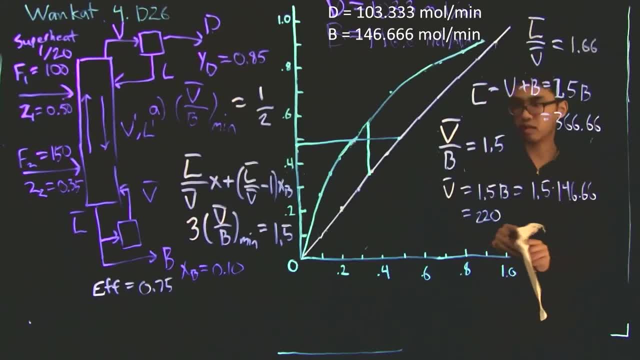 1.66.. And so now we can trace the operating line. So it's going to once again start from 0.10.. And it's going to approximately run from 0.10 to 0.4 and 0.6.. 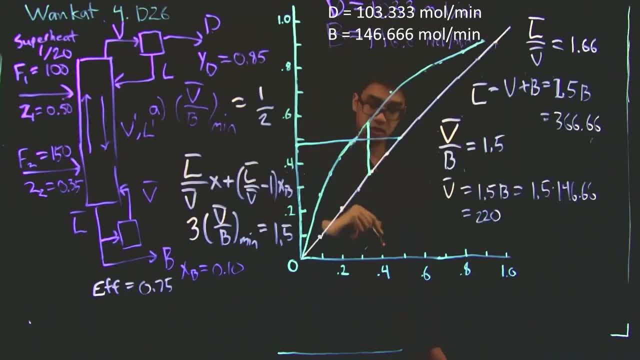 So this would be here, And so our operating line is going to look something like this. Next step is to calculate the intermediate operating line between the bottom operating line and the top operating line. This one uses the flow rates v-prime and l-prime. 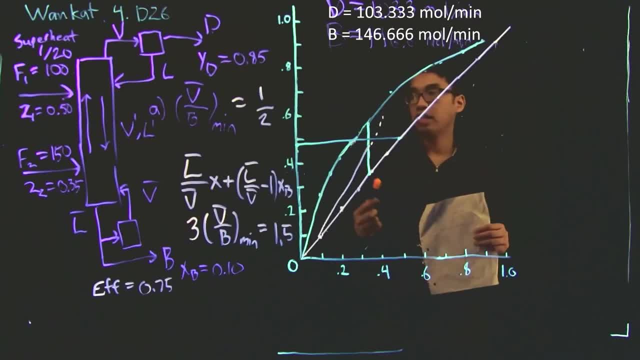 so we need to calculate that. We can do that by taking into account the mass balance at the feed tray of the saturated liquid, which is this operating line. So if we look at it, we'll see that the liquid v-prime is coming in. 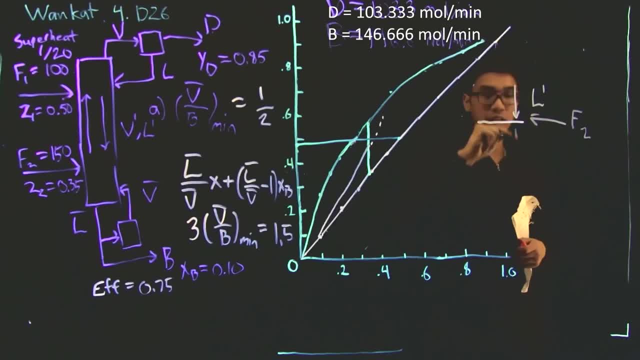 We have the feed, F2.. Then we have liquid l-bar. We also have v-bar and v-prime. Since the feed is completely saturated, we know that l-prime is plus. F2 is equal to l-bar. That means that from mass balance, 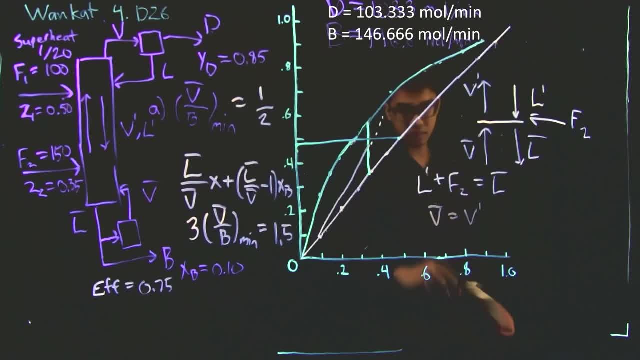 v-bar is equal to v-prime. So we have l-bar and F2.. And so l-bar minus F2 is equal to l-prime. l-bar is 366.66 minus 150 is equal to 216.66.. So the l-bar 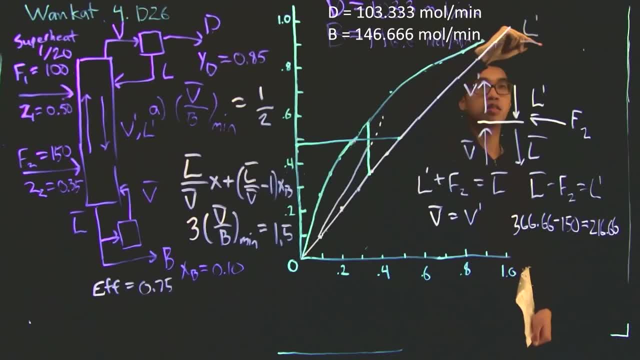 the l-prime over v-prime ratio is equal to 216.66 over 220,, which is equal to 0.984.. And so on this graph, it would be almost parallel with the xy-line, but with a slightly smaller slope. 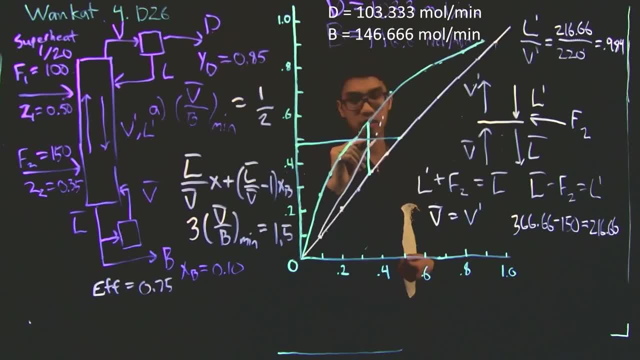 And so it would look something like this. And so the intersection point is here. Now the third operating line. we could calculate it by calculating the flow rate at the top of the column, But we don't need to do that because we know that it has to pass through the point 0.90..